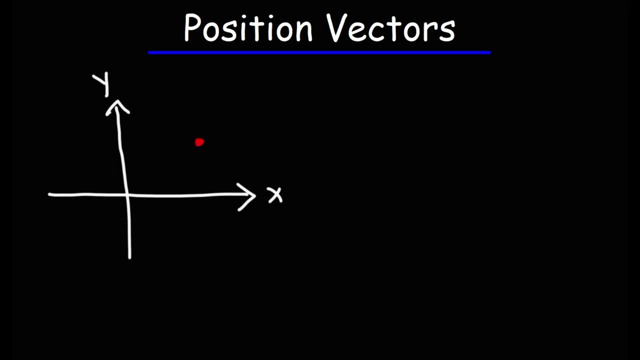 And let's put a point on this graph. We'll call this point P, which is at 3,2.. Now to draw the position vector. we're going to draw it from the origin to the point of interest. So that's the position vector. 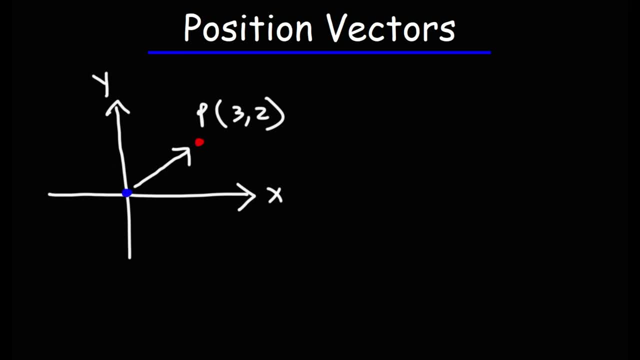 It's a vector that starts from the origin and points to a particular point. It's represented by the symbol R with the vector symbol attached to it. Now the origin is at 0.. To write a vector between two points, it's simply the difference in the x values and the difference in the y values. 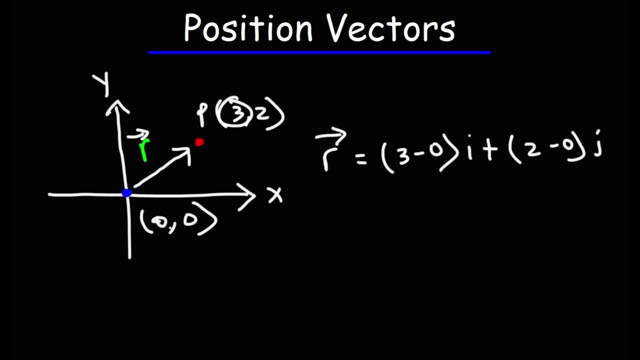 So I'm subtracting 3-0 to get the x component of the vector, And then I'm subtracting the y values 2-0, to get the y component of the position vector. So the position vector for this example is 3i plus 2j. 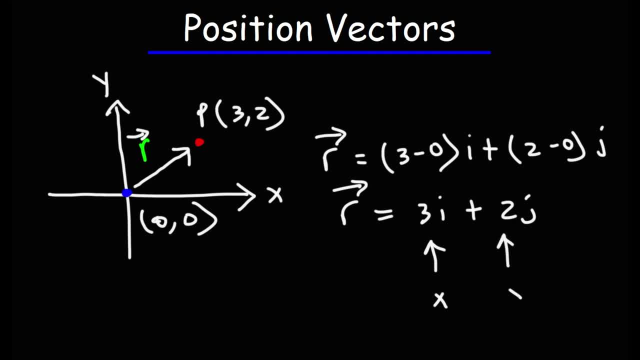 So this is the x component and this is the y component of the position vector And you can see that visually. To go from the origin to point P, we need to travel 3 units along the x direction and 2 units along the y direction. 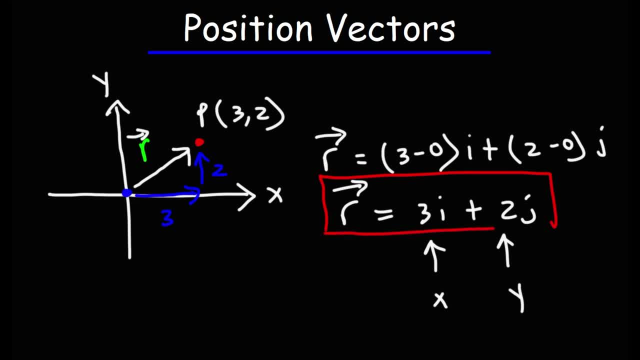 And so we can see why it's 3i plus 2j. So that's how you could find the position vector. Remember it starts at the origin and it's directed towards the point of interest. Let's try another example, but with a 3D coordinate system. 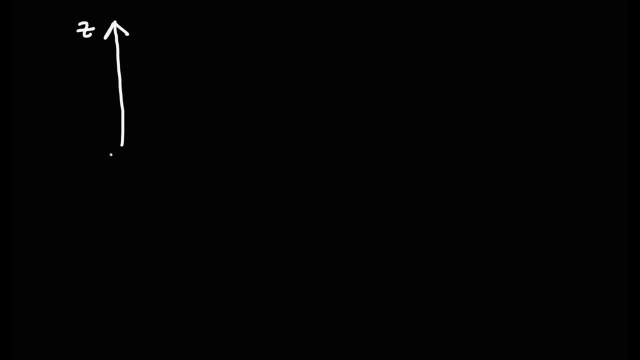 So let's say this is the z-axis. We'll say this is the x-axis And this is the y-axis. Now let's say we have some point P. We have some point P which is at 3,, 4,, 5.. 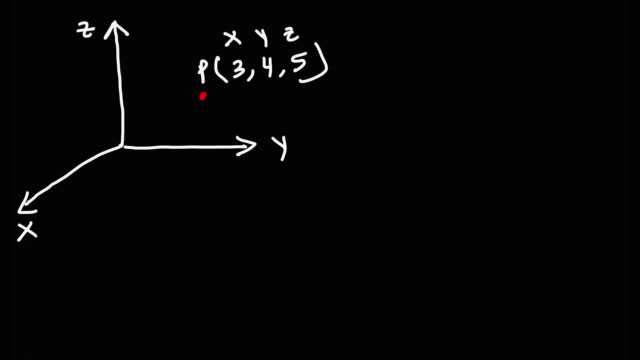 So this is x, y, z. So to get to that point, starting from the origin, we need to travel 3 units along the x direction and then 4 units along the y direction, and then up 5 units along the z direction. 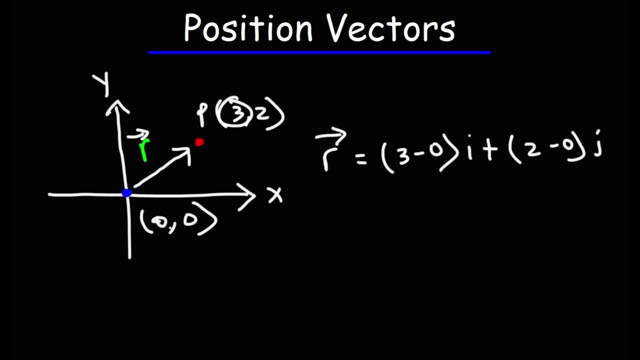 So I'm subtracting 3-0 to get the x component of the vector, And then I'm subtracting the y values 2-0, to get the y component of the position vector. So the position vector for this example is 3i plus 2j. 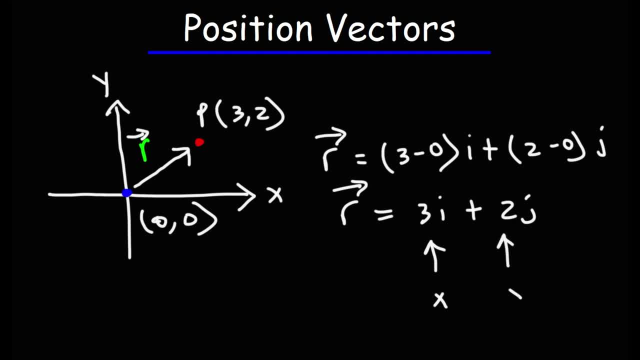 So this is the x component and this is the y component of the position vector And you can see that visually. To go from the origin to point P, we need to travel 3 units along the x direction and 2 units along the y direction. 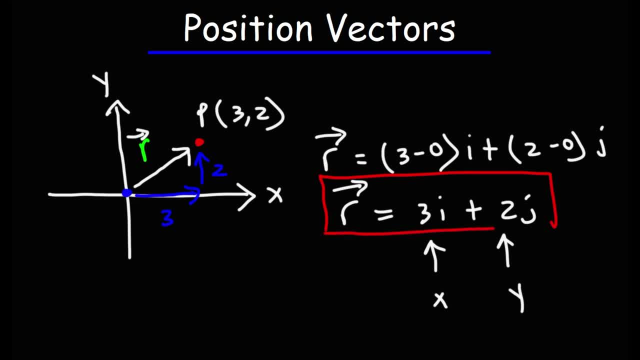 And so we can see why it's 3i plus 2j. So that's how you could find the position vector. Remember it starts at the origin and it's directed towards the point of interest. Let's try another example, but with a 3D coordinate system. 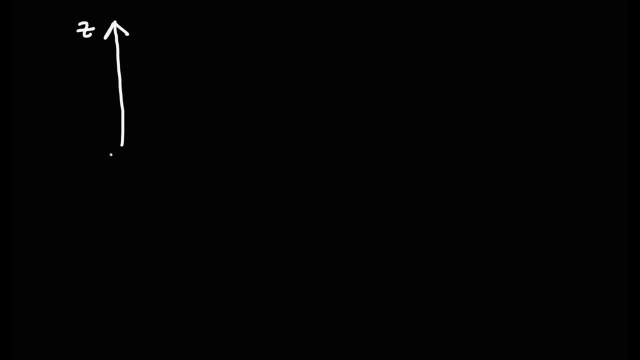 So let's say this is the z-axis. We'll say this is the x-axis And this is the y-axis. Now let's say we have some point P. We have some point P which is at 3,, 4,, 5.. 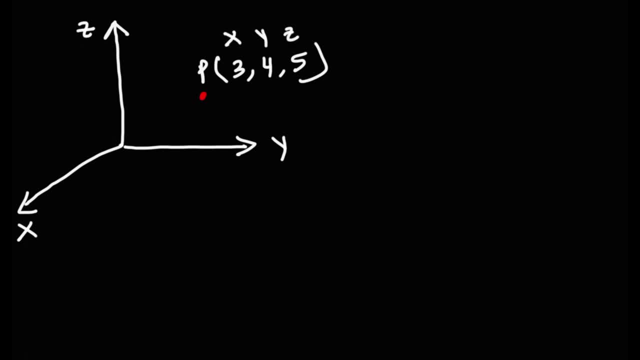 So this is x, y, z. So to get to that point, starting from the origin, we need to travel 3 units along the x direction and then 4 units along the y direction, and then up 5 units along the z direction. 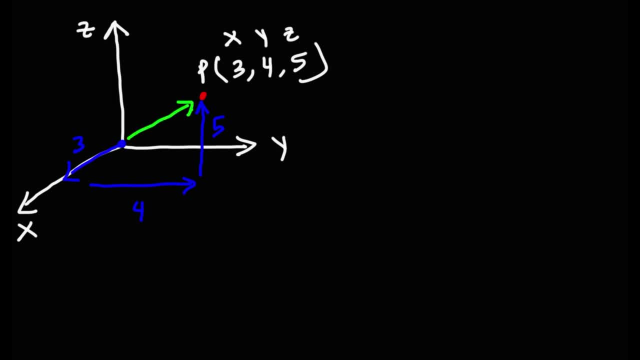 So here is our position vector R. So it's going to be 3i plus 4j plus 5k. Now here's a question for you: How can we determine the length of the position vector R? How long is this position vector? How long is this position vector? In order to determine the length of the position vector R, we need to determine the length of the position vector. In order to determine the length of the position vector R, we need to determine the length of the position vector. 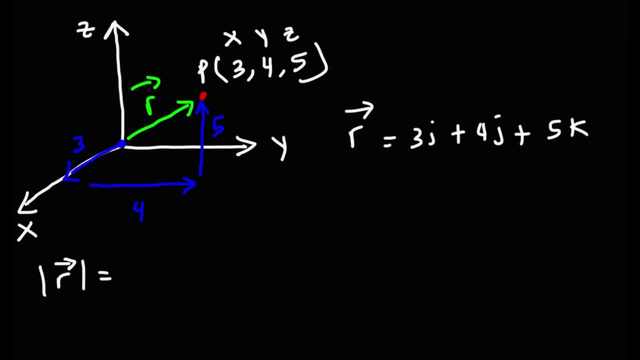 You're basically finding the magnitude. Now, if it's for a 2D coordinate system, it's going to be the square root of x squared plus y squared. But for a 3D coordinate system, like the example that we have, it's going to be also plus a z squared inside of a square root symbol. 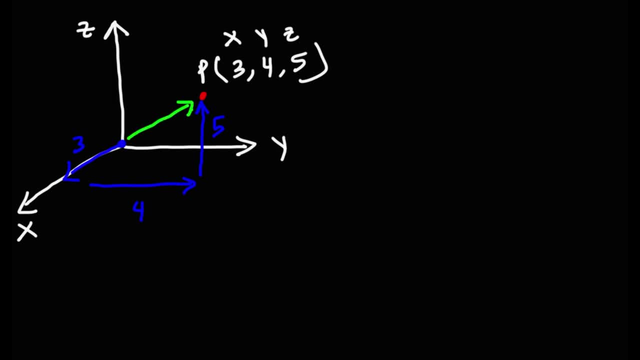 So here is our position vector r. So it's going to be 3i plus 4j plus 5k. Now here's a question for you: How can we determine the length of the position vector r? How long is this position vector? 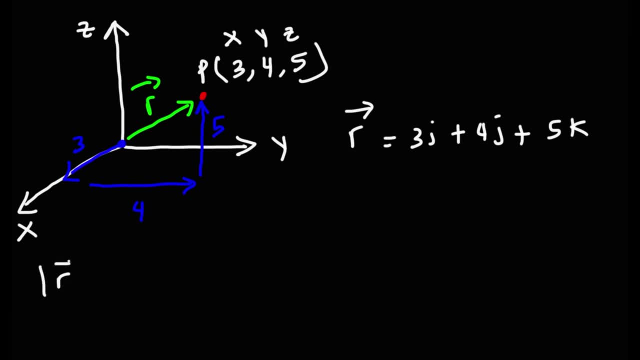 In order to determine the length of the vector r, we need to find the length of the position vector r, the length of the position vector. you're basically finding the magnitude. now, if it's for a 2d coordinate system, it's going to be the square root of x squared plus y squared, but for a 3d, 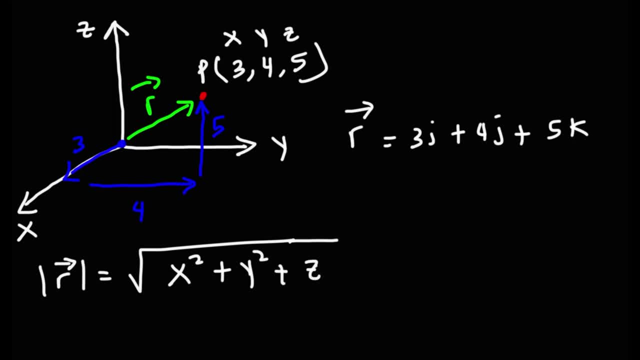 coordinate system. like the example that we have, it's going to be also plus a z squared inside of a square root symbol. so for this problem it's going to be the square root of 3 squared plus 4 squared plus 5 squared. 3 squared is 9, 4 squared is 16, 5 squared is 25.. 9 plus 16 is 25, 25 plus 25 is 50.. 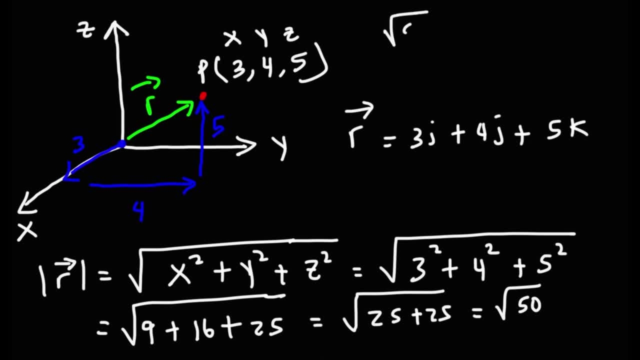 so we have the square root of 50, which we can reduce. that 50 is 25 times 2 and the square root of 25 is 5.. so is the magnitude of the position vector, which is also the same as the length of the position vector. 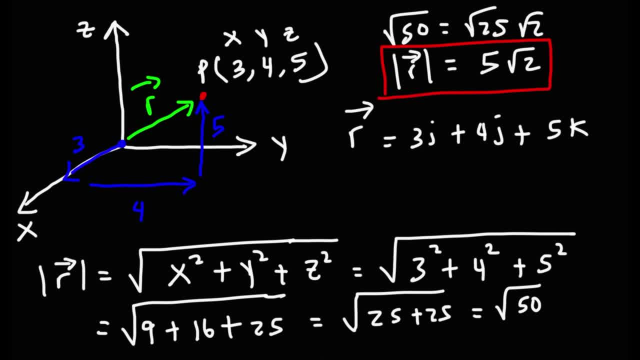 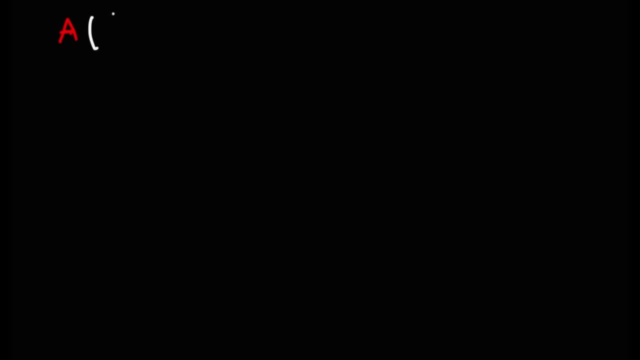 so that's how you could find the length of any vector really. now let's say we have a particle that moves from point a, which is at 2 comma, 3, comma 4, and it's going to move to point b, and let's say that point b is located at 5. 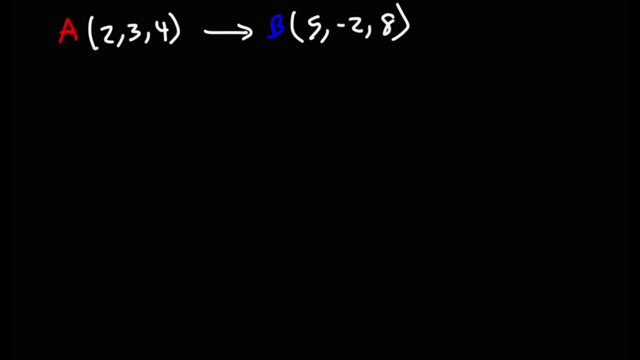 negative 2, 8.. so for this problem, find the position vectors that point to point a and point b and then use those position vectors to calculate the displacement vector as the particle moves from point a to point b. now to find the position vector for point a, it's simply going to be 2i plus 3j plus 4k. 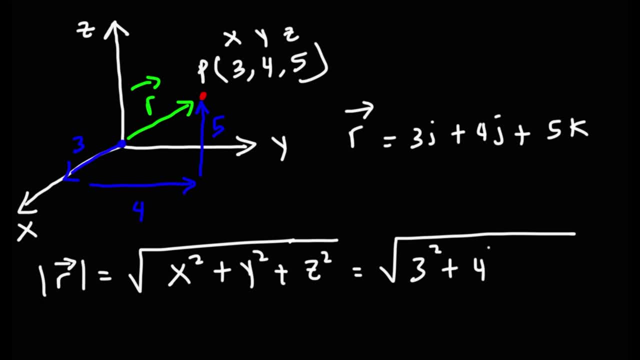 So for this problem it's going to be the square root of 3 squared plus 4 squared plus 5 squared. 3 squared is 9,, 4 squared is 16,, 5 squared is 25.. 9 plus 16 is 25.. 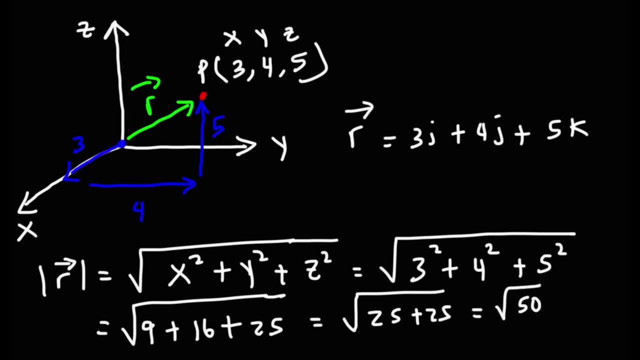 25 plus 25 is 50. So we have the square root of 50, which we can reduce. that 50 is 25 times 2. And the square root of 25 is 5.. So this is the magnitude of the position vector, which is also the same as 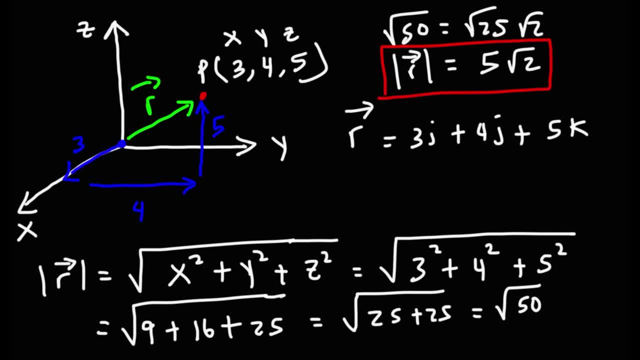 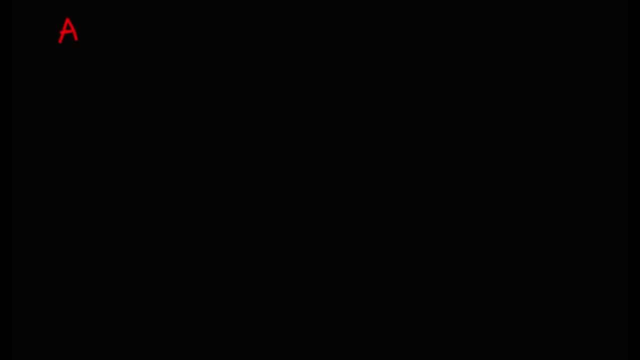 the length of the position vector. So that's how you can find the length of any vector, really. Now let's say we have a particle that moves from point A, which is at 2,, 3,, 4. And it's going to move to point B. 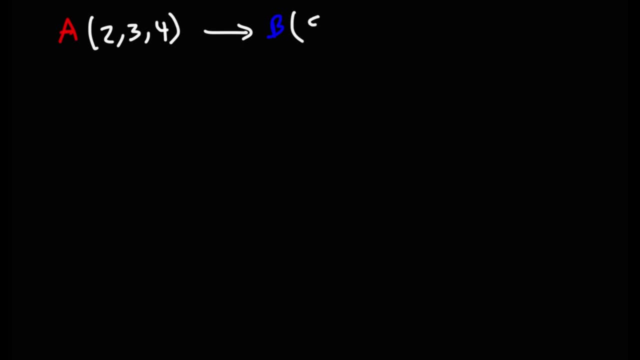 And let's say that point B is located at 5, negative 2, 8.. So for this problem, find the position vectors that point to point A and point B And then use those position vectors to calculate the displacement vector as the particle moves from point A to point B. 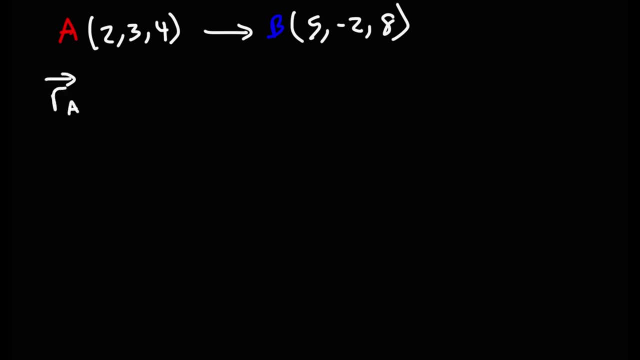 Now to find the position vector for point A, it's simply going to be 2i plus 3j plus 4k. To find the position vector for point B, it's simply 5i minus 2j plus 8k. 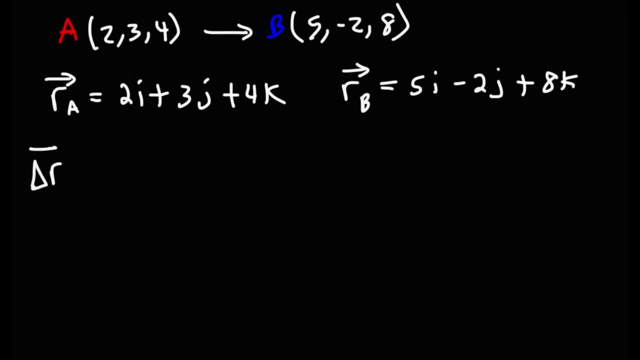 Now to calculate the displacement vector using the position vectors. it's going to be the difference between the two. So as we go from A to B, initial to final, it's going to be the final position minus the initial position. That gives us displacement. 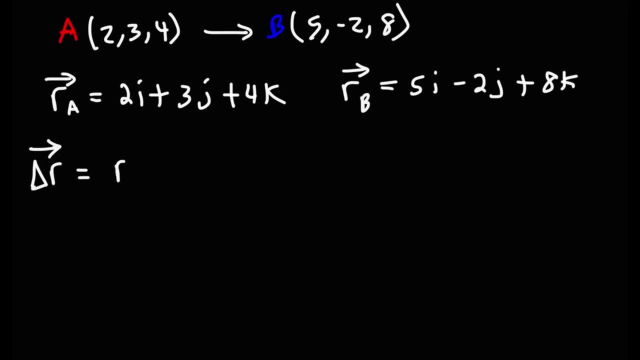 Displacement is the change in position. So we're going to take r and b and subtract it by r a And that's going to give us the displacement vector, If we take the final position vector minus the initial position vector.